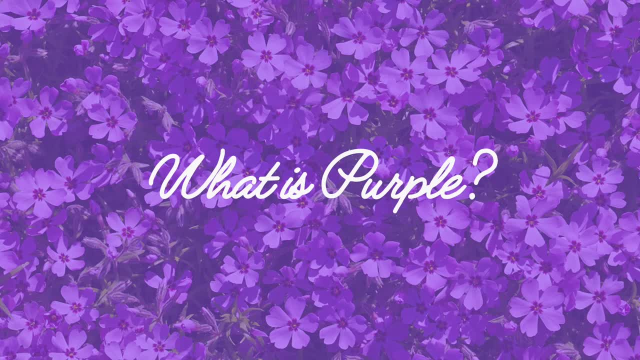 the color itself. Purple is a blend of red and blue. It's often used interchangeably with violet, but there is a slight difference: Purples have more red in their blend versus violets that have more blue. The first use of purple is actually found in prehistoric cave art. One example of 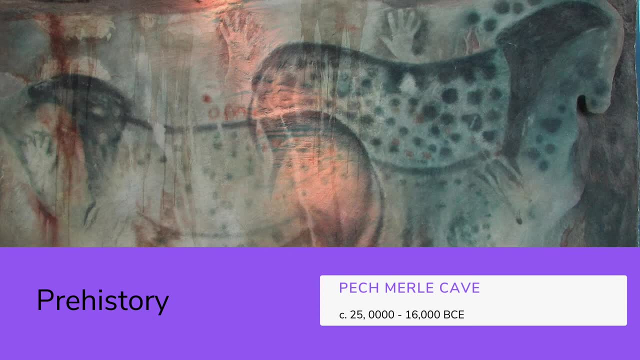 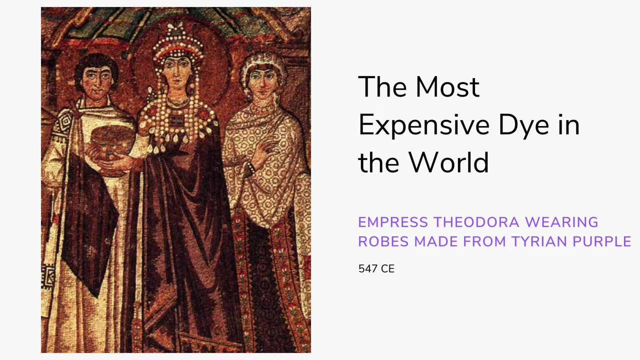 this is the Pecmerle Cave in France, dating from between 25,000 and 16,000 BCE. Early humans would blend manganese and hematite powder to create pigments that would be used to paint animals, handprints, outlines and geometric shapes. In ancient Greece, purple became highly prized. This. 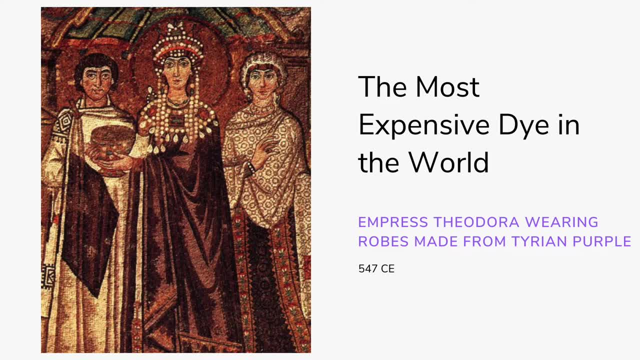 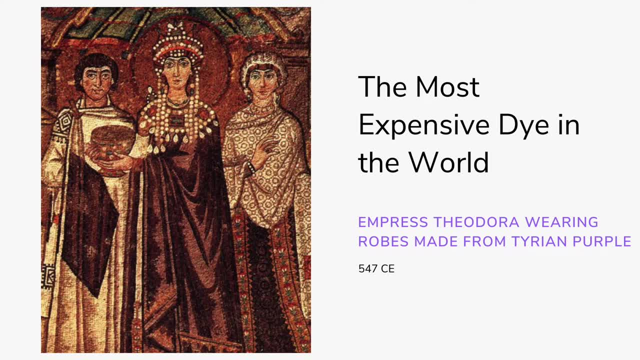 a technique was developed to create a purple dye. It was named for the city and called Tyrian purple. A process involved opening the shells of thousands of Bolonus brandaris snails. Then the snail's mucus would be exposed to the sun. After a while it turned a vibrant reddish-purple that adhered to. 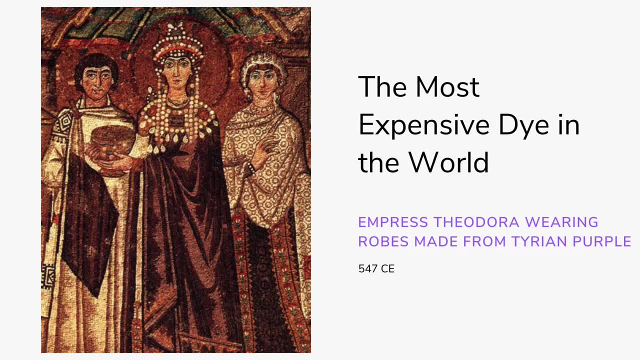 fabric incredibly well. However, it would take about 250,000 snails to make a single ounce of dye. Even today, archaeological excavations are still uncovering mounds of discarded snail shells. Because of this tedious process, Tyrian purple was extremely expensive. This is how the color. 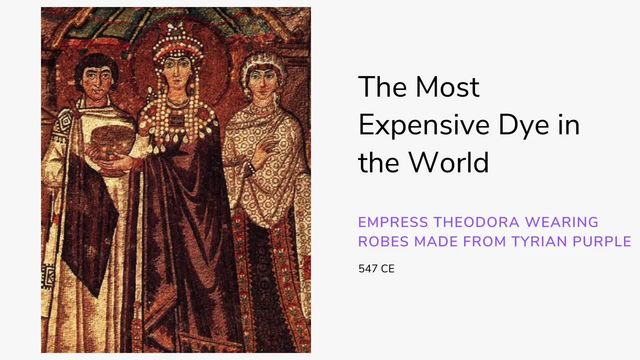 became associated with the noble class and royalty because they were the only ones that could afford it. In fact, 4th century BCE, historian Theopompus wrote that quote. Tyrian purple was used up until the end of the 15th century when the Byzantine Empire fell to. 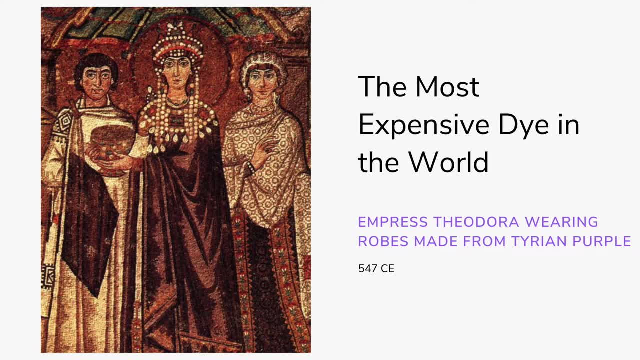 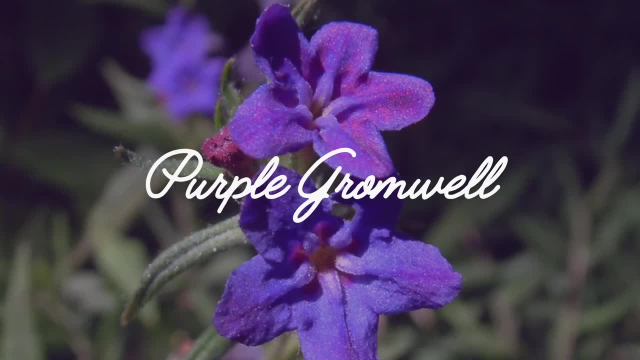 the Ottoman Empire. In fact, that's what forced the Catholic Church to change the cardinal uniforms to red. There just wasn't any purple left. In China, purple dye was used for clothing, but it was made with a plant: purple gromwell. 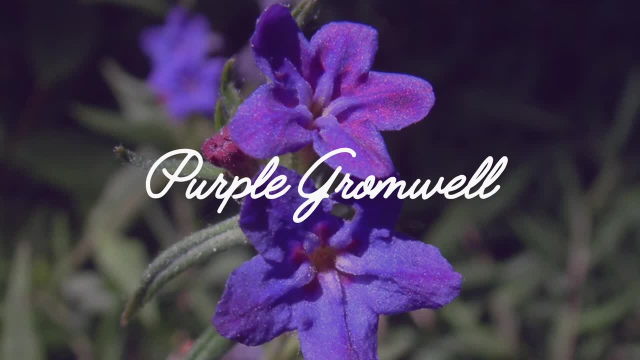 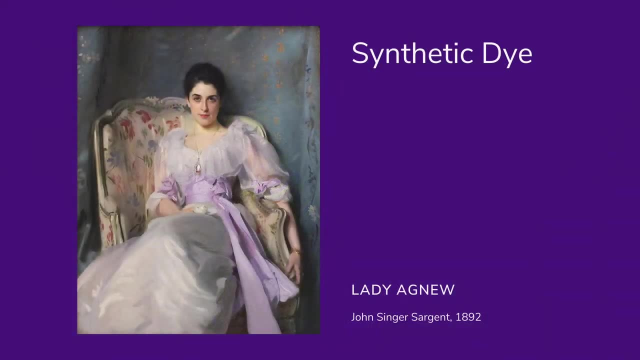 instead of snails. Interestingly, purple wasn't as highly prized in the East as it was in the West. It was seen as a secondary color, but was still used in clothing and art. It wasn't until 1856 that a synthetic alternative was discovered. That year.